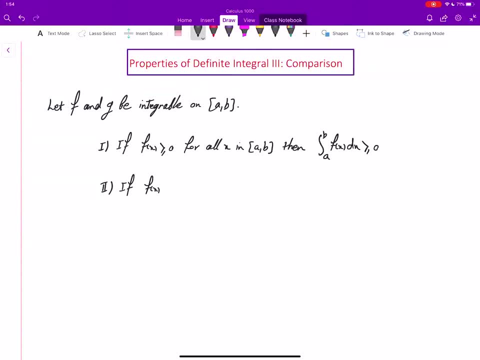 that if a function is bigger than equal another function, for all x's in the interval a- b, then the integral of the bigger function is going to be bigger than integral of the smaller function. In other words, the function, the integral, definite integral, is increasing functional in some way. 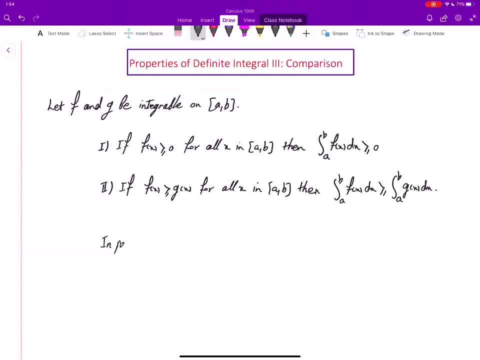 And while, in particular, if we know that a function f of x is between two numbers, for all x in the interval a- b, so if we know that the function is between, let's say, absolute mean here absolute max M, then integral of function, that function is between absolute doc and absolute max capital M. 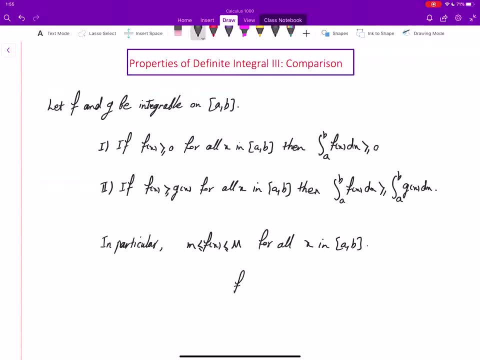 will be better. So that will be k, i, which is the integral of function a. b was correct, Then integral of Helen Ceylon. We didn't Chris, that function could not be correct. We can take the integral wherever the normal function, isasing fromaria. if we know that the function is between, let's say, absolute mean here, absolute max, capital, m, yes, then integral of this lambda muss be. and plus m, plus become integral of this lambda. If we look here, he is again pretending to understand the integration of all x by that. Hold on for two arguments. when we Xi Don Juan derriere, R, if we look at every function f of x, 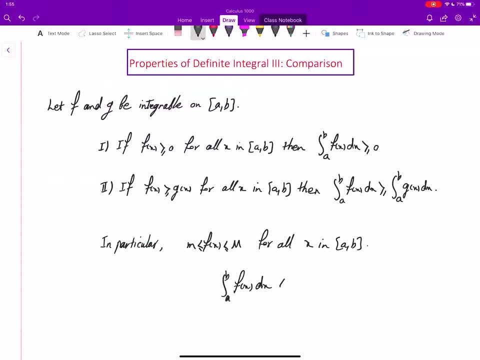 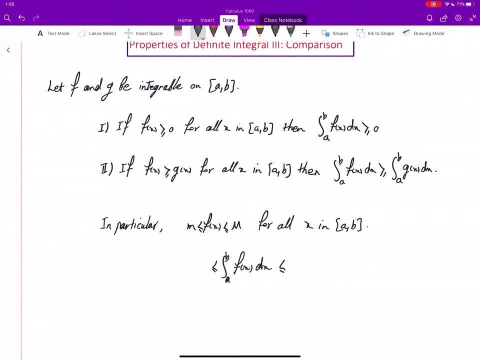 from a to b can be approximated by integrals of these constants. you see, this is going to be integral of m a to b dx and this is going to be integral of lowercase m dx, a to b. well, uh, we know that if you have a constant, you look at the area there. uh, the region is going to 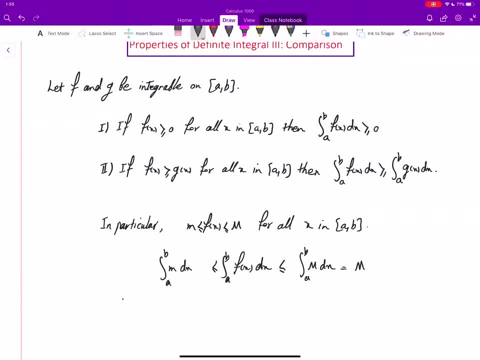 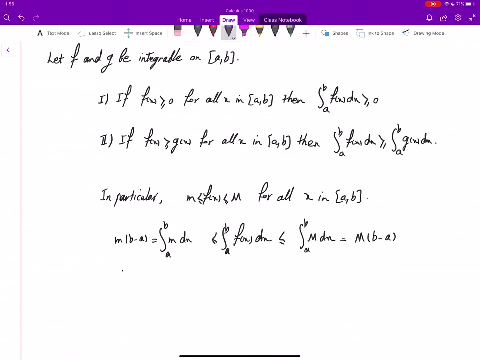 be rectangle, and while either positive, negative m doesn't matter, it will be the area of that or the, the width times, m, and this guy is going to be m b minus a. and while seeing these, uh, these properties is not difficult, i will just go ahead and do one thing: someone. 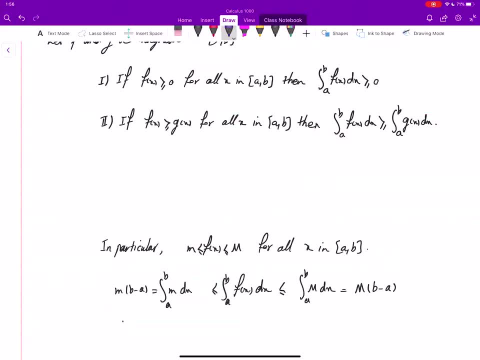 graph for the second one. you see, if i have two functions, let's say both of them are positive, in this case, um, this is f and oh. oh, we are supposed to have g less than f. okay, this is f. f is above uh, g. then, from the uh, on the interval a to b, the uh integral of g dx is going to be the region of. 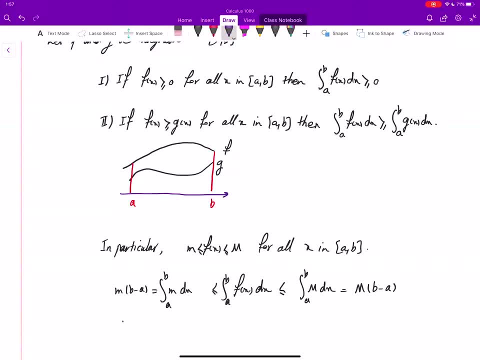 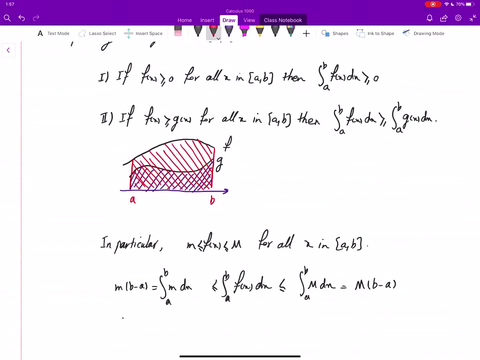 the, the area of the region, this piece here, and it is obvious that this is less than the area of the get bigger function, and that's how you show that the second property, which is, by the way, equivalent to the first property, is true. okay, let's see how this works. i will just go ahead and do one thing. 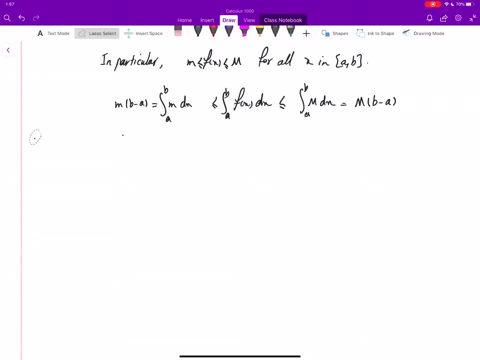 some examples here. uh, the last thing, that the last property that we saw there can be useful to estimate some of the functions. meaning what? meaning that i don't know how to compute this integral now, but i know that sine squared x is between: uh, what sine x itself is between 1 and. 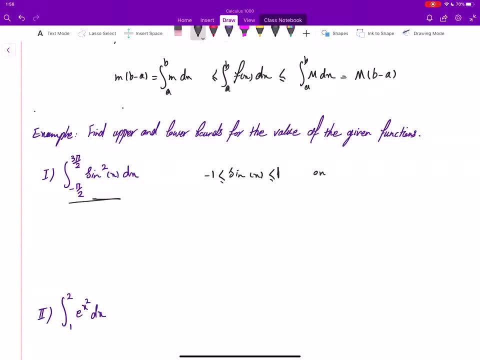 negative 1 on the interval negative pi over 2 and 3 pi over 2.. if you square that, this is going to be a number between 1 and 0. square is always positive. yes, now, from using the last property that we saw here, integral negative pi over 2, 3 pi over 2, which i 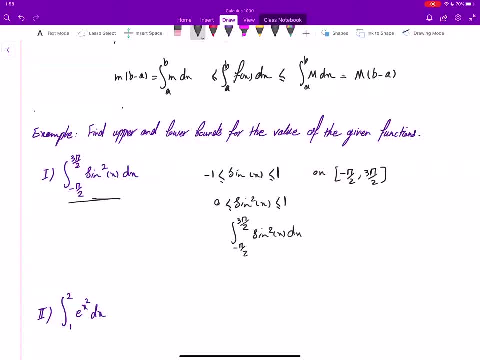 don't know how to compute that, so i'm going to use the last property that we saw here. compute yet is going to be less than 1 times 3 pi over 2 minus negative pi over 2, and it's going to be greater than 0 times b minus a. 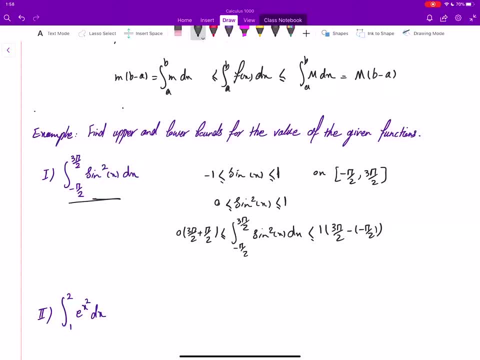 which is this. so, in other words, the integral of sine, squared from negative pi over 2 to pi, is going to be between what? 4 pi over 4, which is 2 pi and 0. it will be a number over there, so i don't know what is the exact number, but i can definitely say that 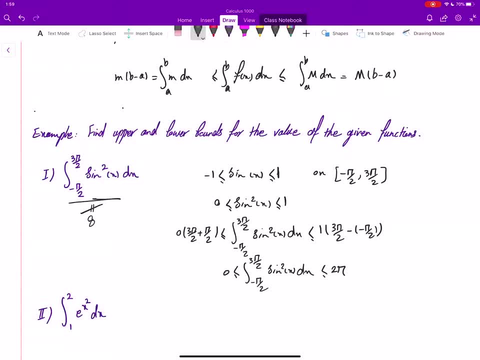 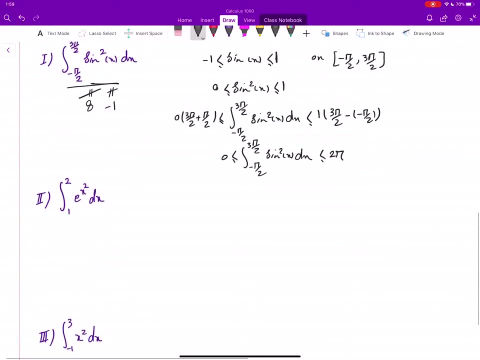 it's not going to be a number like 8. it's not going to. it is between 2 pi, which is 6 point something, and 0, and it's not a negative number. definitely can say that. how about this one? well, we have e to the power x squared, the best approximation you can get. 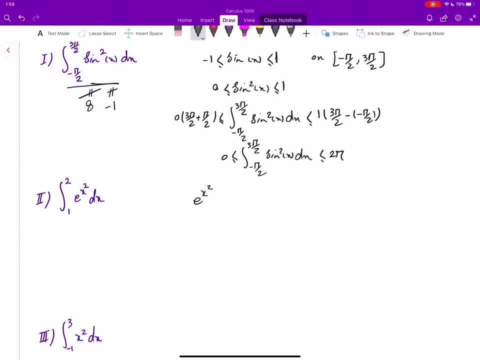 here is using absolute max and mean on the interval. so on the interval one and two the absolute max max is e to the power 4 and The absolute power медpay, 그러면 a to the new mean value of internship. so it is 1 plus 0. 0. So here we have thebag product in here, And theout line was니까- and it had two detriments- 1 plus 1, which is 3 plus 3, and all those is equal to 1.. Alright, you get the às in here now. now, all these are equal to 4, so you think there. 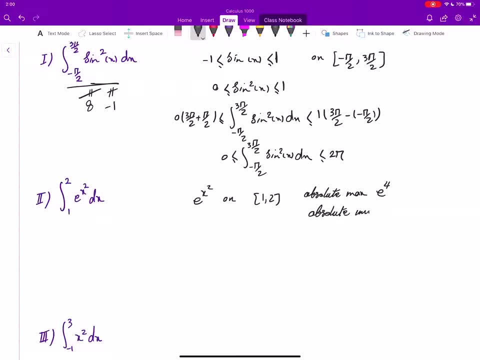 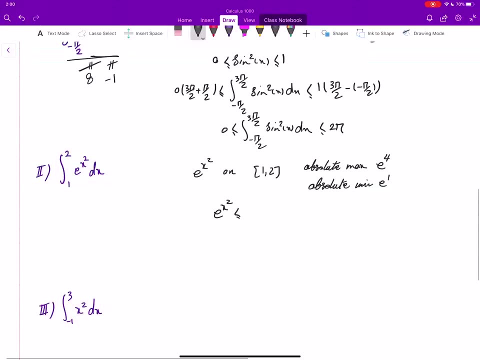 absolute mean is e to the power one, So in other words e to the power x squared. the function is between two and one. then we can use the property, the integral of that. oh sorry, not two and one. e to the power one and e to the power four on the interval one, two, Then e to the power x squared. 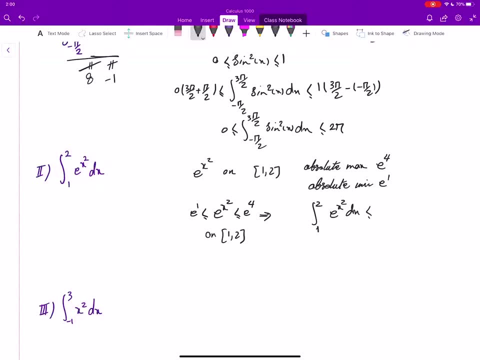 dx is going to be between e to the power four, two minus one, and e to the power one, two minus one. From this we know that the value of e to the power x, squared dx from one to two, is a number between e to the power four.